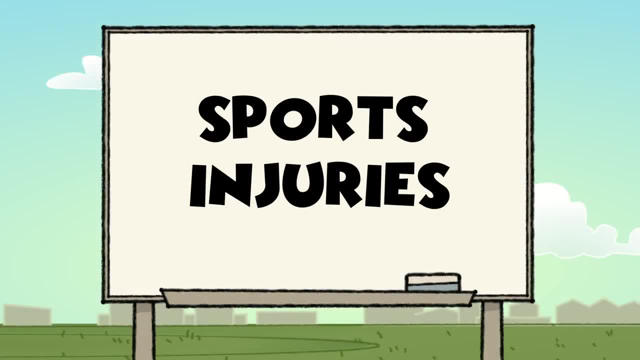 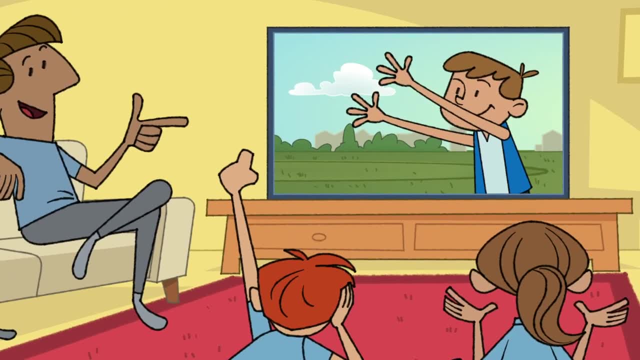 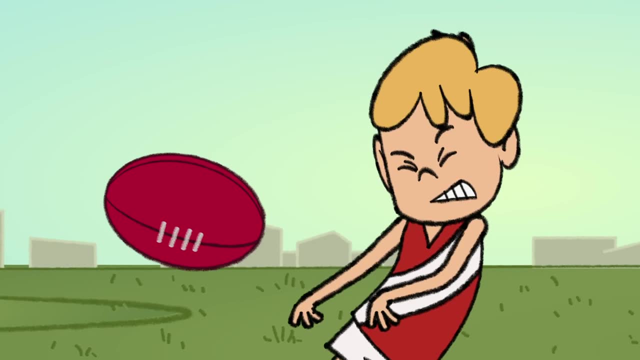 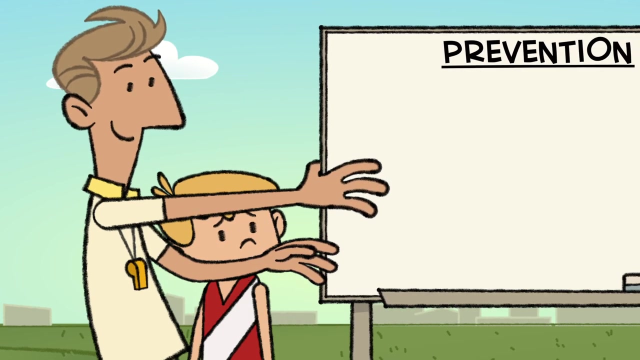 In Australia, the only thing we love more than watching sports is playing sport, But, as any parent knows, wherever there's running and other physical activity, there's also the potential for injury. That's why we're here: to coach you on ways to prevent and treat injuries, plus recognising 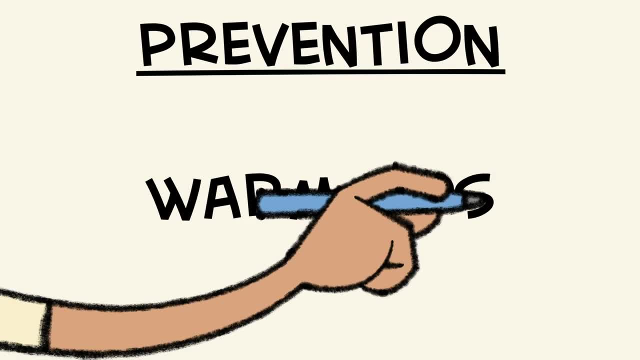 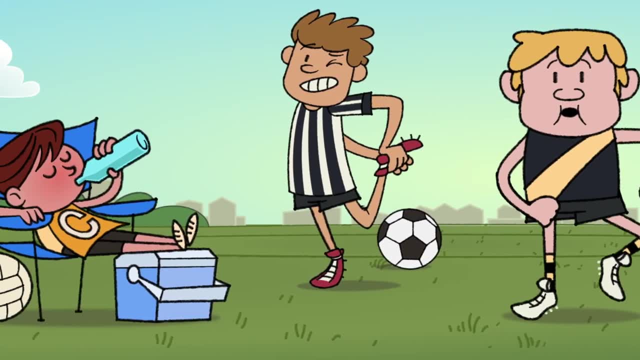 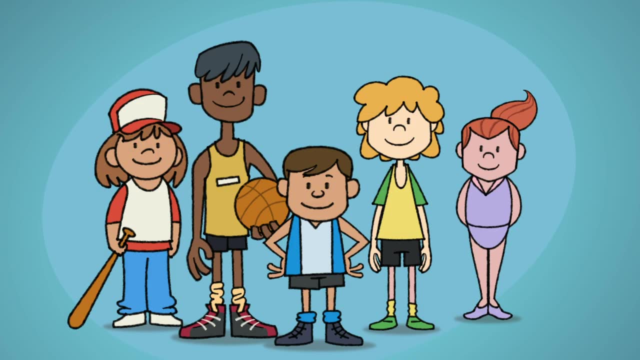 certain conditions. And to get you warmed up, let's start with an easy one: warm-ups At the start of any training or game. it's important to warm up by jogging and stretching. Likewise, it's important to cool down too. It's no secret that kids grow fast and the difference one year. 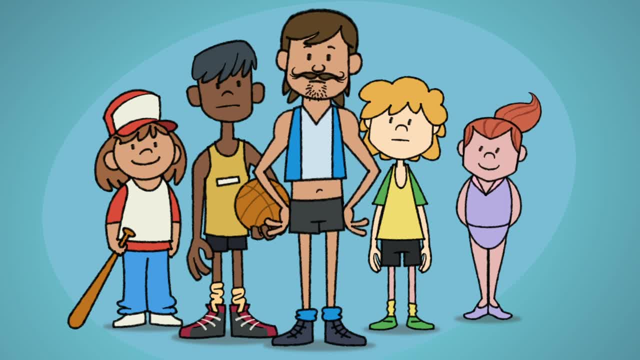 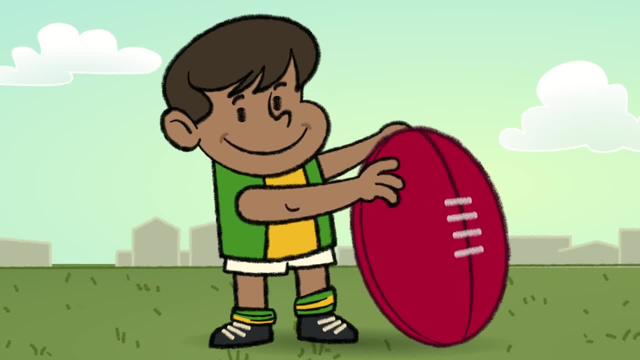 can make is huge. That's why you need to make sure your child is enrolled in sport that's appropriate for their age and skill level. You should also consider modified sports like Auskick, depending on your sport equipment, Helmets, mouth guards, padding and proper footwear can. 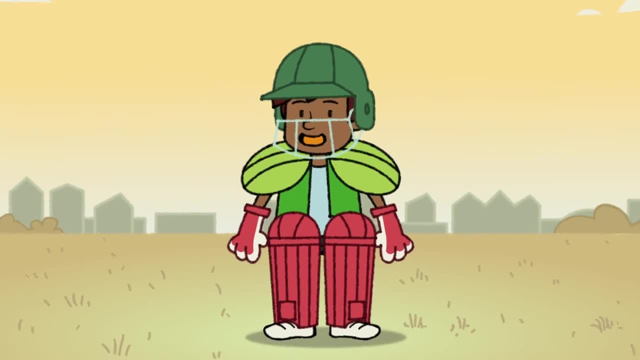 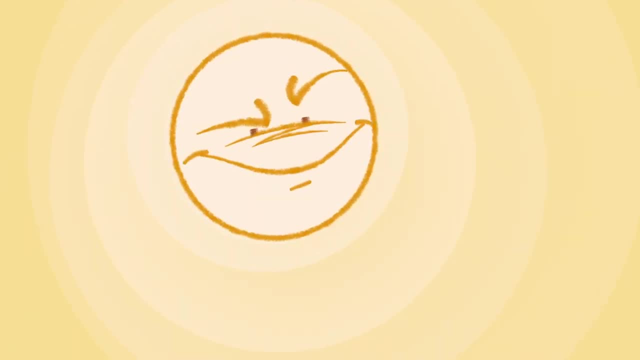 prevent or reduce injuries And, while you're at it, remember to protect them from the sun as well. Unfortunately, it's not just people who like to come and watch sport. this guy does too, And when the sun's out, there's an increased risk of dehydration and heat-related illnesses. 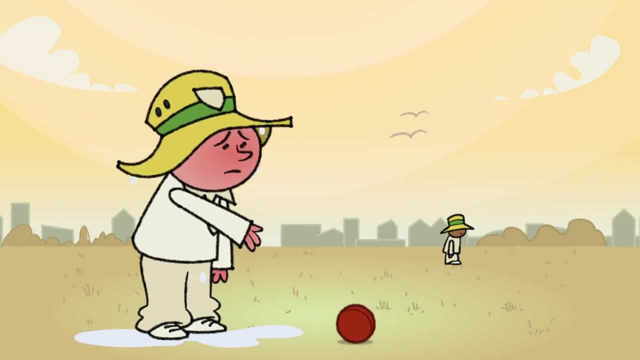 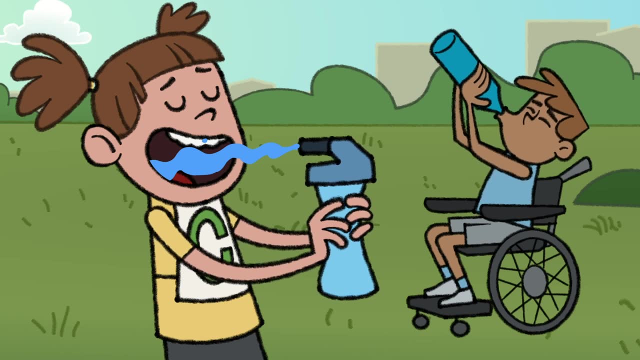 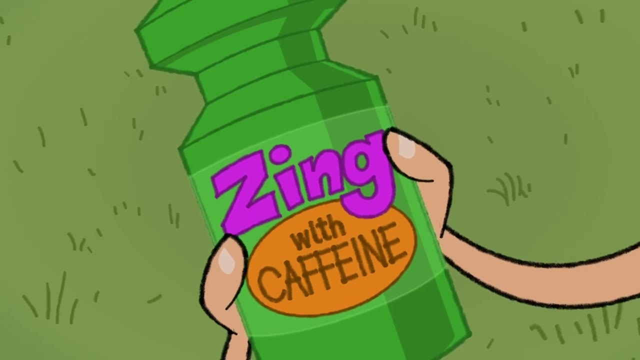 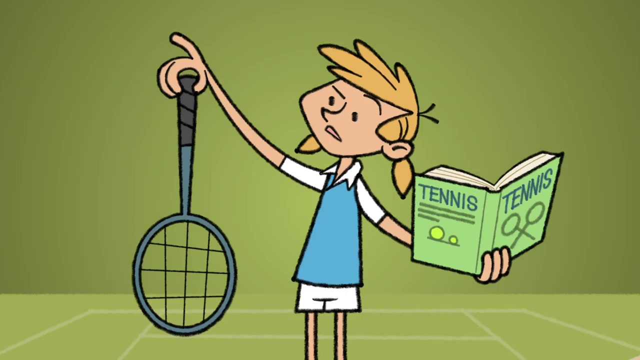 especially in sport where exposure is prolonged, like crickets and long-distance running, Cool water is the best choice for children to stay hydrated. High-calorie sport drinks are generally unnecessary for most children participating in sport, and energy drinks with caffeine should be avoided at all times. This is an important question Before a 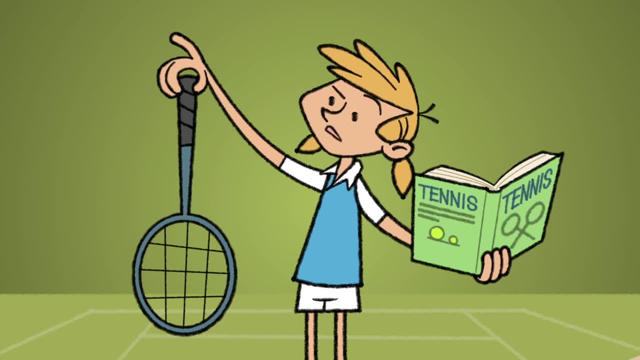 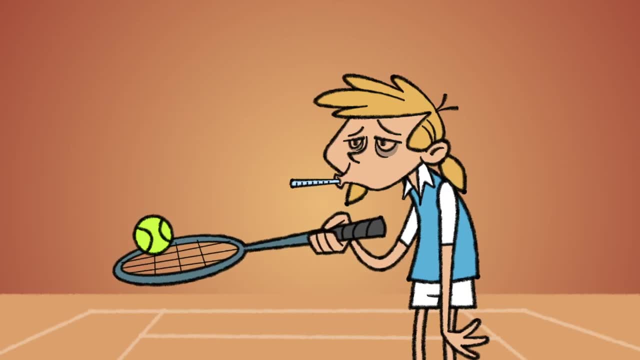 child participates in a competitive game. they should participate in training to learn and develop their skills. Plus, you should make sure they're not tired, ill or injured, and should they be in good shape. If the child is in a bad condition, the coach should be informed about it. 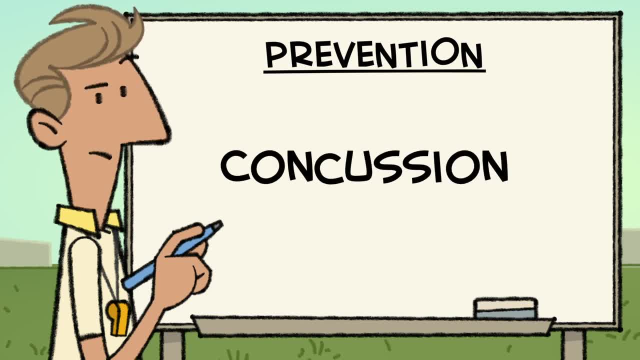 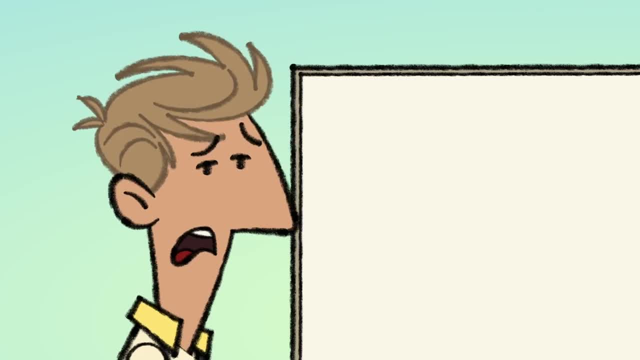 A concussion is a mild brain injury which can occur from contact with another player equipment or the playing surface. But what you might not know is that symptoms may not show until hours after the incident. So it's important to watch out for warning signs like the sufferer may have.